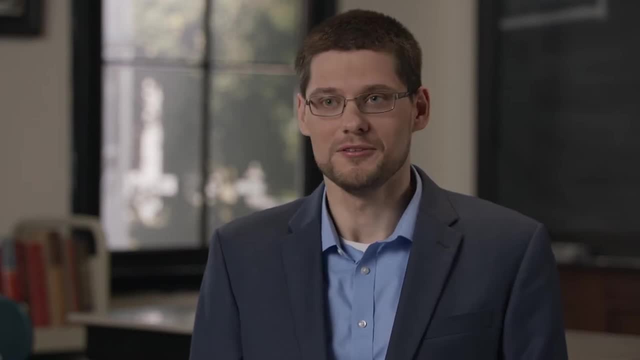 teaching them how they can be lifelong healthy individuals without that regular, daily reinforcement. These exercises also need to be age appropriate. I just mentioned push-ups. Push-ups are not something most kindergartners are capable of doing, at least not well And frankly. 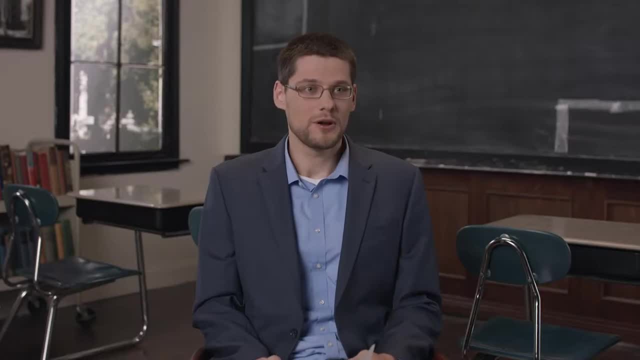 at that age they don't have the upper body strength to do it. And third, off, we want to choose exercises which are going to expand the child's physical abilities. So in grammar years there's a certain lack of coordination in the child. 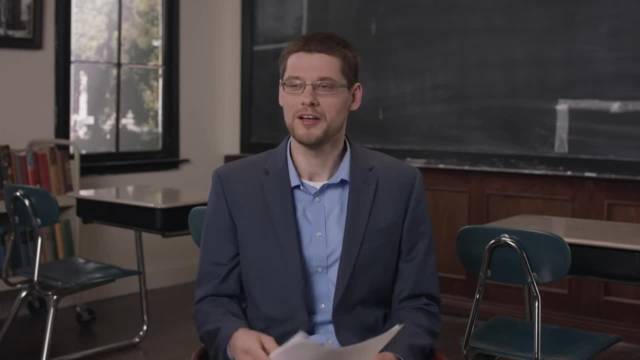 They don't know how to use both sides of the body to attain one goal. They run slightly awkwardly. So these are things we're going to emphasize at that point, because they have certain abilities already in place and we want to take those abilities and grow them. 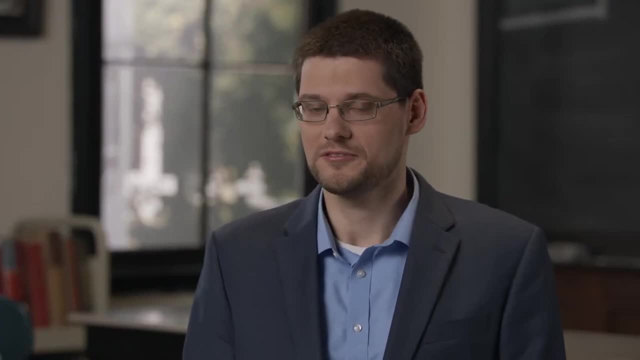 over time. Last point, perhaps the more important point on what physical education is, is that it's an arena in which we can practice virtue. We know that fatigue is a thing which makes us want to quit. Our body says no, I'm done, I don't want anymore. But part of being virtuous. 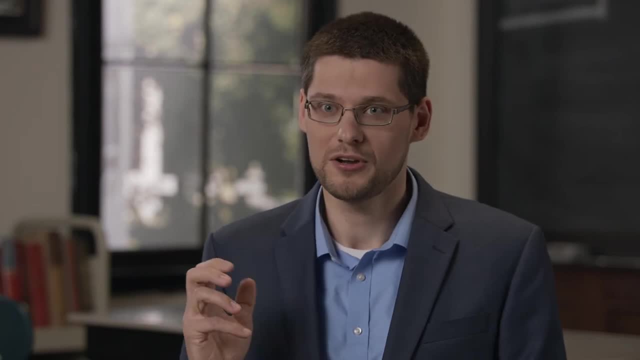 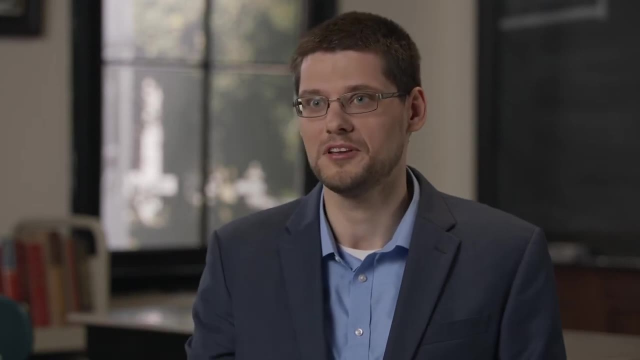 is overcoming that, building a strong, having a strong mind in approaching this so that we can do that one more push-up, We can hold the plank for 15 more seconds, We can sprint the final 10-meter stretch in our quarter-mile run. And then, of course, competition, Competition. 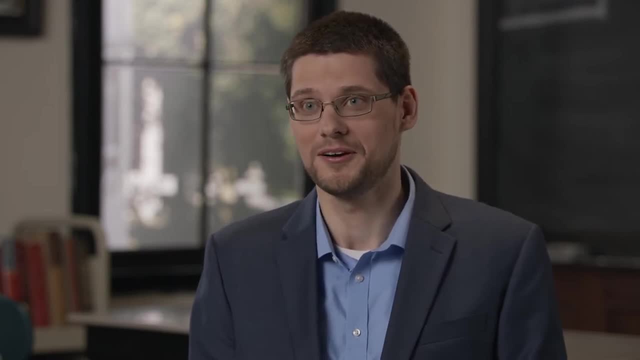 brings out many vices, especially in the young. because they want to win. So they're willing to cheat the rules because they think the teacher isn't looking or no one will notice, And then when they're accused they will lie about it, And in a physical education class. 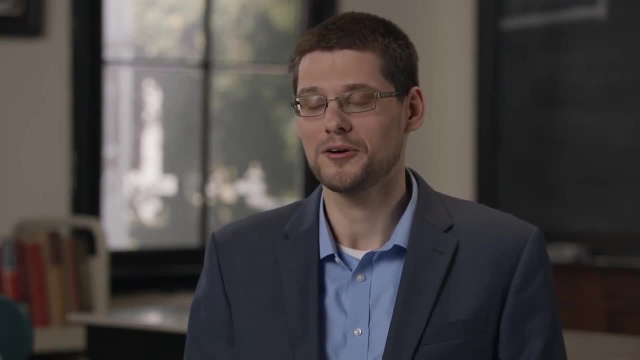 we take those things very seriously. These are matters of justice, of right and wrong. So we need to correct these students and we need to teach them, encourage them to play these games fairly, so that they can all enjoy them that much more. 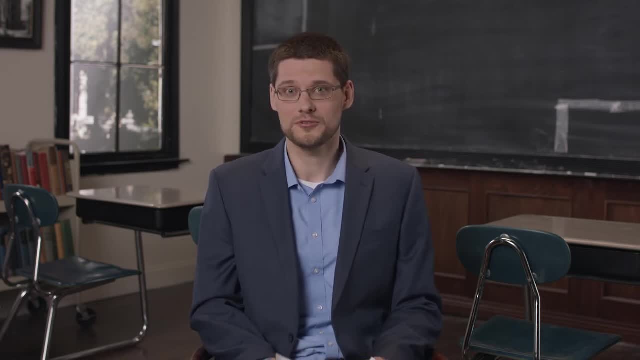 Parents, I want to share a few ideas of what you could do to reinforce your child's physical education at home. And the first one perhaps won't be as popular, but I think we can all admit that we don't exercise as much as we ought to. There's a rare individual who actually 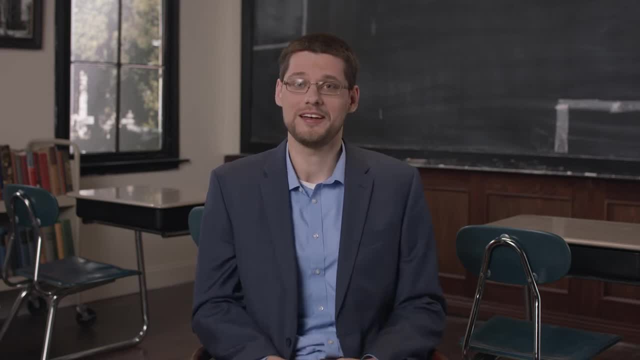 who does? I think we can answer that and say honestly, I work out as much as a person ought to. So maybe give your child a chance to show off what they do. They come home and maybe on a Saturday morning you ask them to show you. 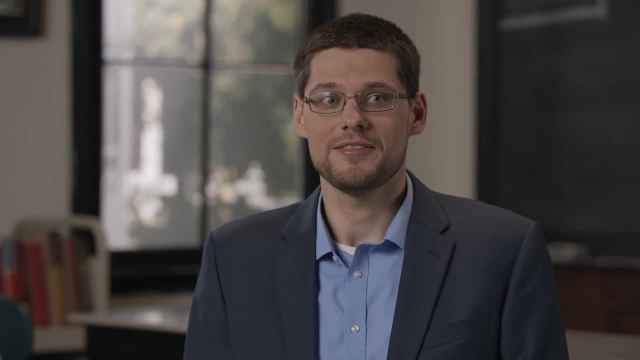 What did you do in particular? What did you do in particular? What did you do in particular? What kind of PE class, What kind of exercise are you doing these days? And then join them for those exercises. Don't let this become a thing where they're the coach and they're 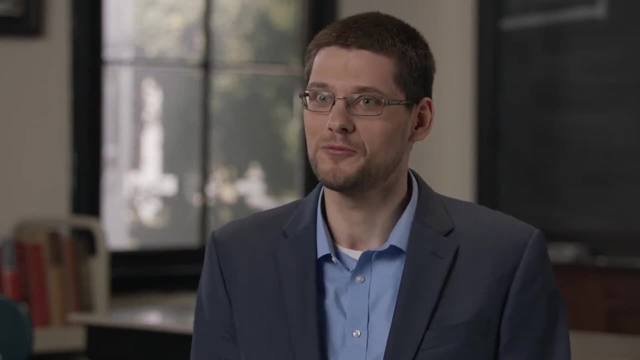 barking at you. you know, do one more pushup. No, you are joining them for this thing And you'll get a little exercise out of this. They'll be motivated and they'll have something to offer at the home and I think everyone will come away pretty well with that. 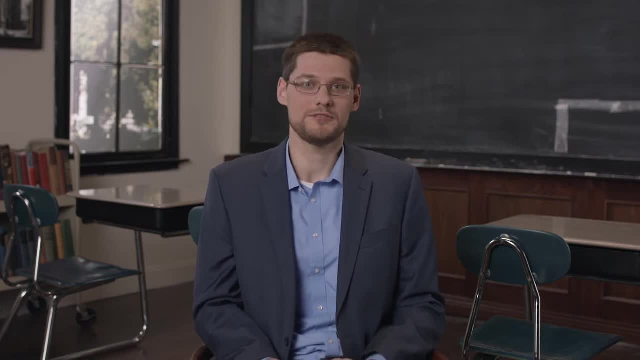 And play games that they're playing in PE. Most physical education classes play seasonal sports, So in the wintertime that's basketball season, Fall that's volleyball and soccer season. So maybe during the course of the year, on those Saturdays, maybe after school. 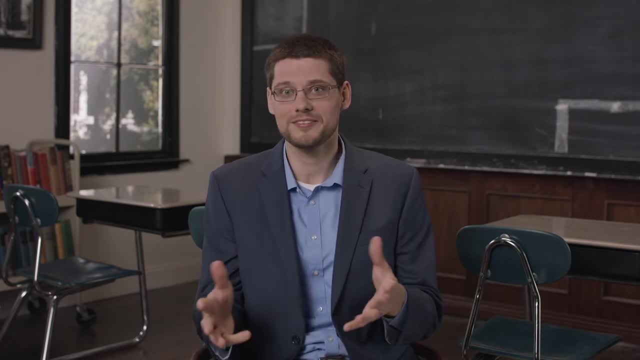 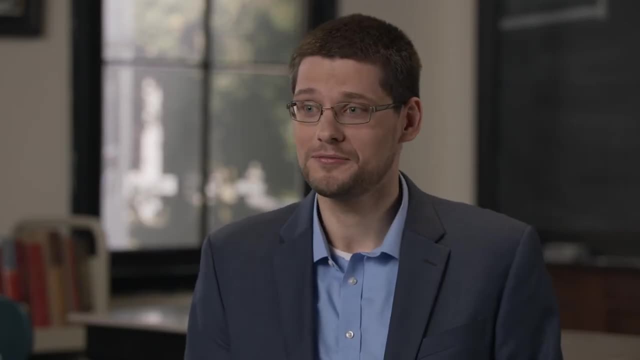 even play those sports with them. If you have a lot of kids at home, send them outside and say: you guys are playing soccer today. Break them into teams and have at it. It doesn't need to be seasonal sports. There are lots of games which we do in PE because we have 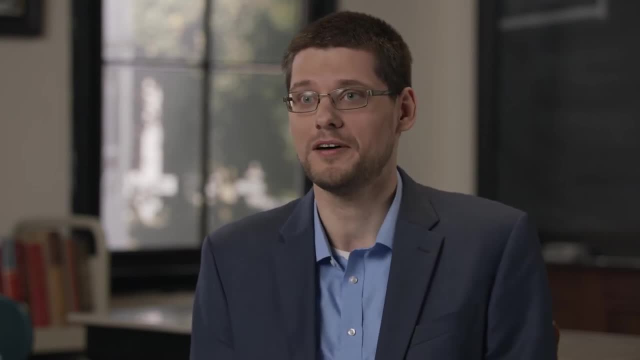 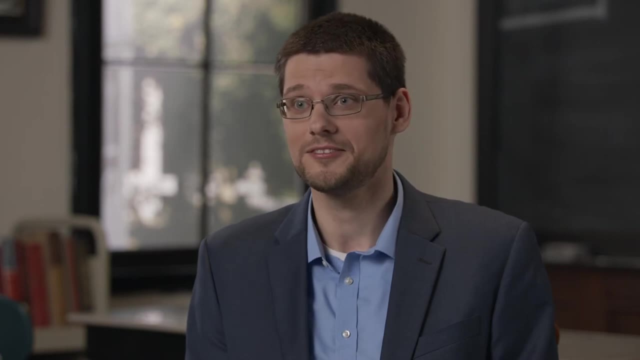 a big group of kids. Some of them can be modified for the home environment. You can do things like your, like play tag. There are countless things that you can do. You can do things that are not in PE. There are countless variations of that. You can do relay races, not just. 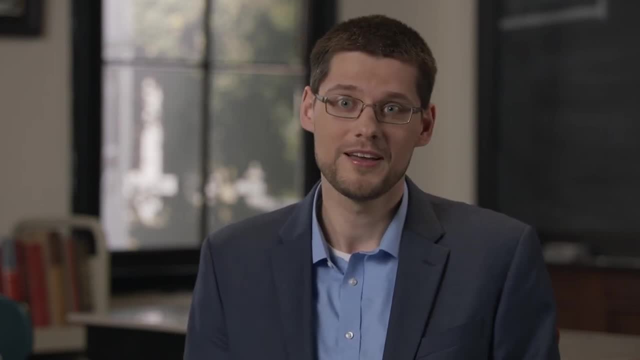 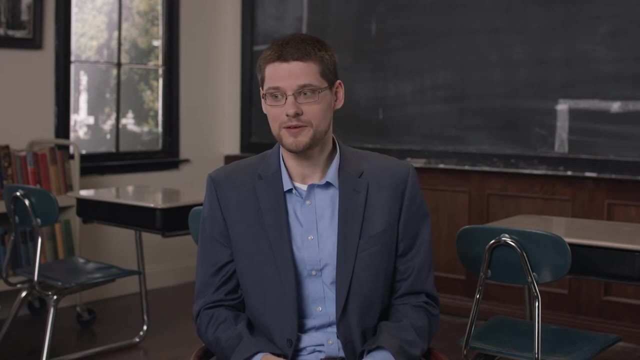 running back and forth across the yard but doing crab walk or running backwards or skipping. So first off, exercising at home. Second thing: teach them to overcome fatigue When you're doing those exercises with them, before or after school or on the weekends. encourage. 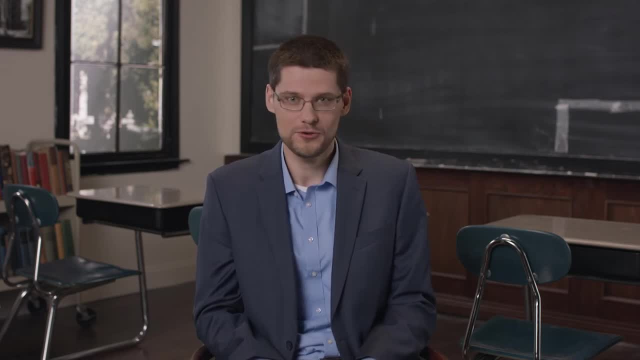 them. Let's do one more pushup right now. Let's hold this plank for a few more seconds, Or, if you have this opportunity- sibling rivalries can be well applied here- Have the siblings compete. Who's going to do more pushups today? Who's going to hold this plank longer? I found 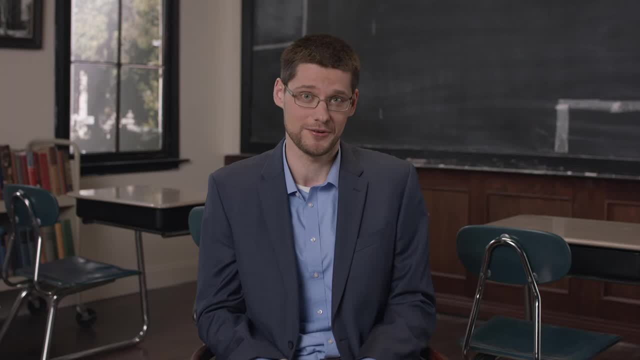 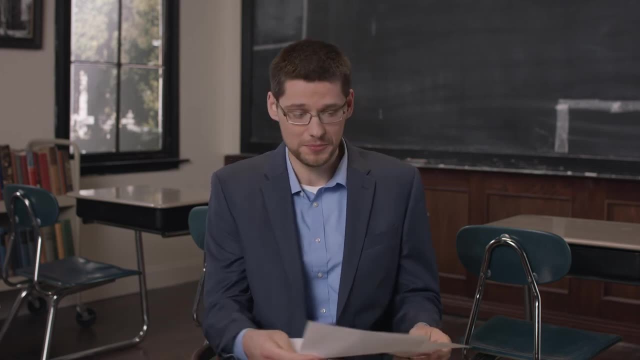 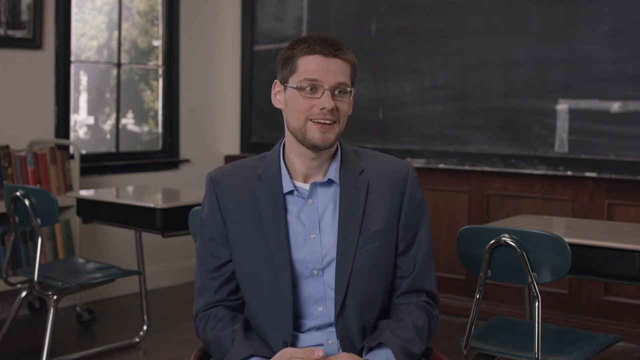 that competition between friends, between siblings, is oftentimes the greatest encouragement, because nobody wants their little sister to beat them, to hold that plank for longer than they did. I mentioned earlier playing sports which are in season, but also be aware that when you play sports at home there's going to be argument. There's going to be, you know. 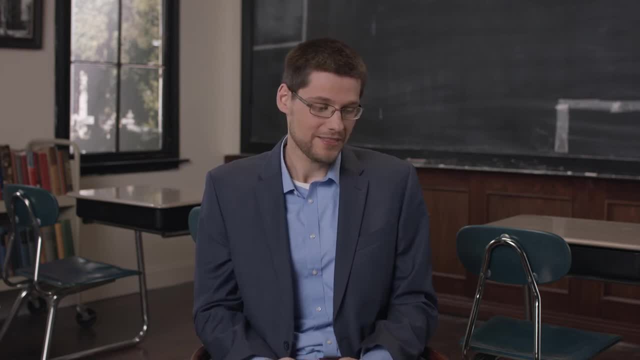 accusations that someone cheated, someone lied, And these need to be treated seriously. So when they come to you asking you to be the arbiter in some disagreement of which you saw nothing, maybe take opportunity to not so much be the arbitrary arbiter but talk. 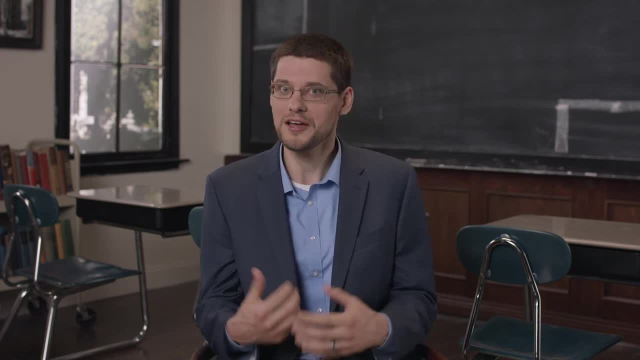 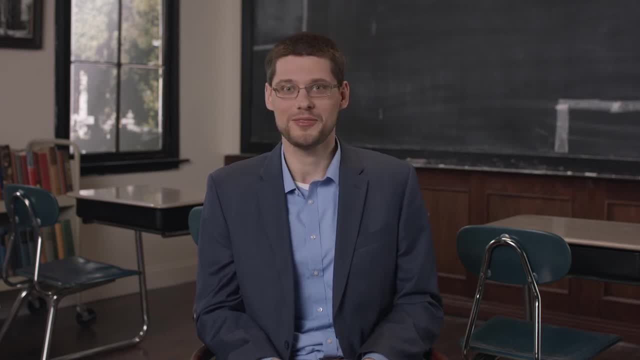 if someone is accusing you of cheating the rules, they know when they're cheating- Or you're seeing another person and then the argument breaks out, ask them: are you guys having fun right now? And I think they will honestly admit they're not having fun. So 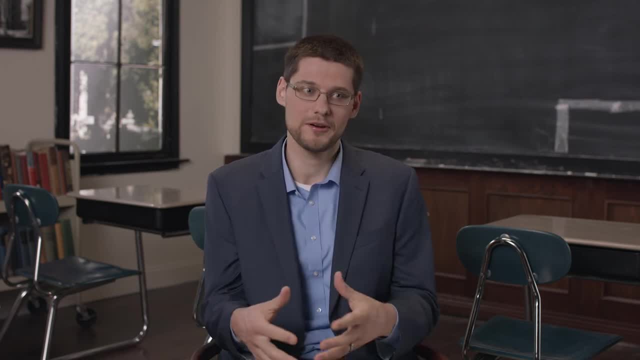 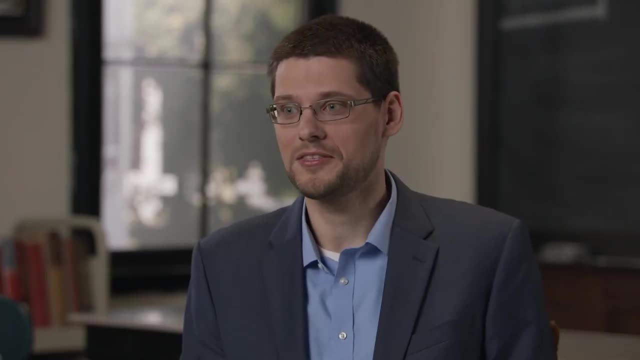 something's got to get, something's got to change. Encourage them to be that fair participant so that we can actually enjoy this game that we do enjoy. Final note, just some toys that I think are applicable to the home environment or any environment. A lot of these are basic. 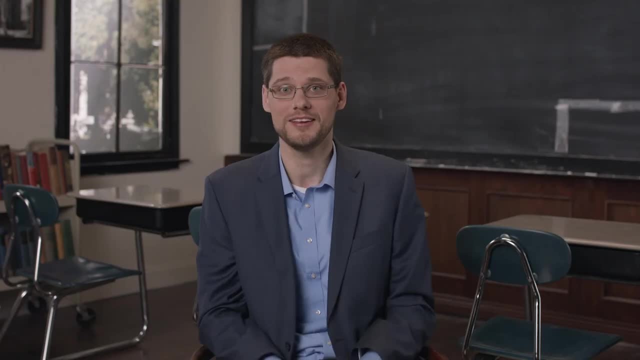 things- Football, soccer, balls, volleyball- have these at home so that kids can make use of them whenever they want to Jump ropes or, even better, double dutch ropes, if you have enough personnel to do those Skip hops. for those of you who know what those are, it's like a ball attached to a 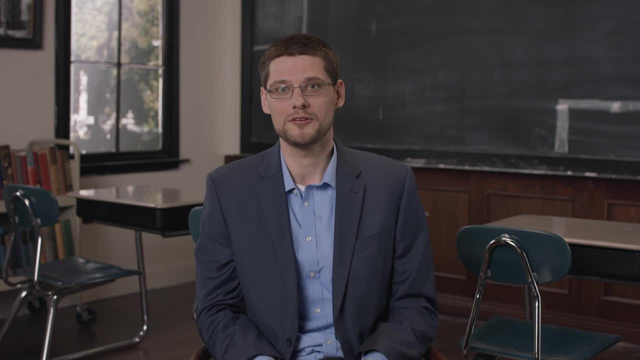 string tied around your ankle which you can spin around your other foot and hop over. It requires minimal coordination, but somehow it's really satisfying because you can get a certain rhythm going with it: An exercise ball, a hula hoop, a tug of war, rope. 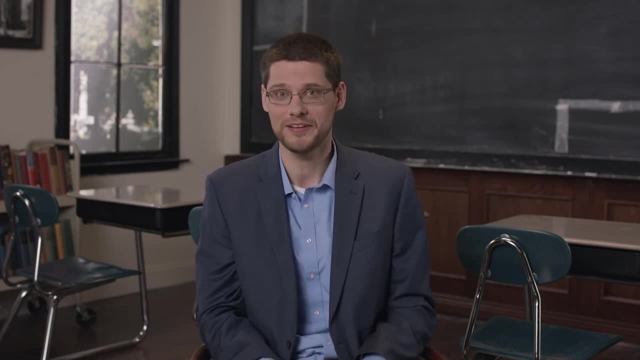 You can do so many things with a tug of war rope. You can do one-on-one tug of war. that's all you have at home And kids love it. You can throw a rope in front of children and say we're going to do this today.